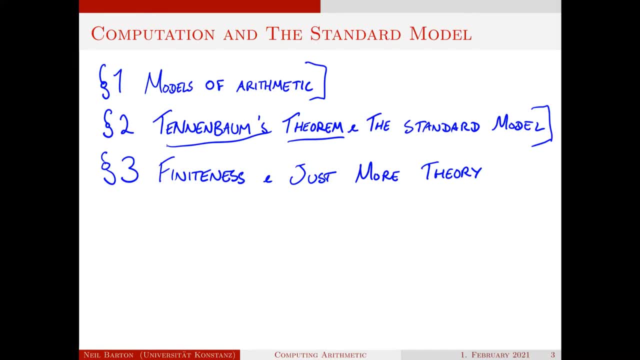 And how people have argued that that might allow us to insulate the standard model. And then in section three we'll consider an objection to this line of argument, namely that this response requires assuming a notion of finiteness which is equivalent to just. 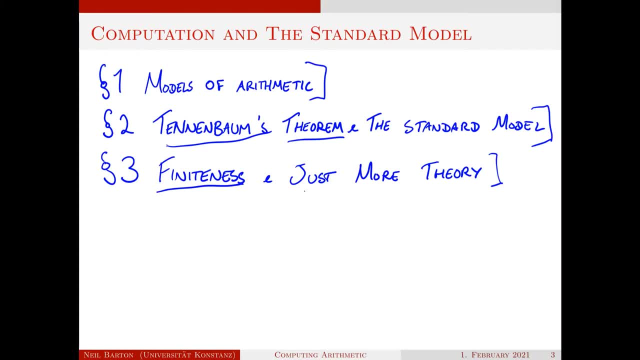 talking about the natural numbers And I'll talk a little bit about how this is situated within the wider context, in particular- And I'll talk a little bit about how this is situated within the wider context in particular- star responses to model theoretic arguments. 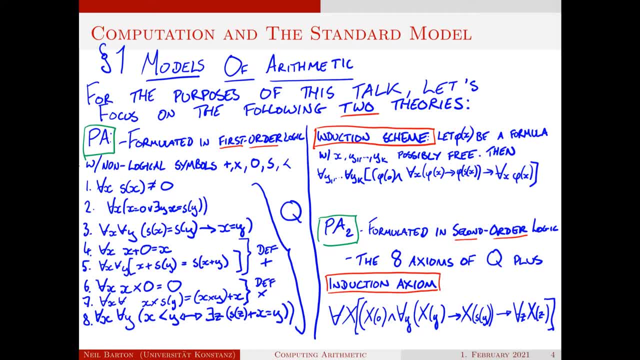 Before we get into the details, let's talk a little bit about the setup here. So for the purposes of this talk, we'll focus on the following two theories of arithmetic. The first is Piano arithmetic- first-order piano arithmetic, and this is formulated in first-order logic right. 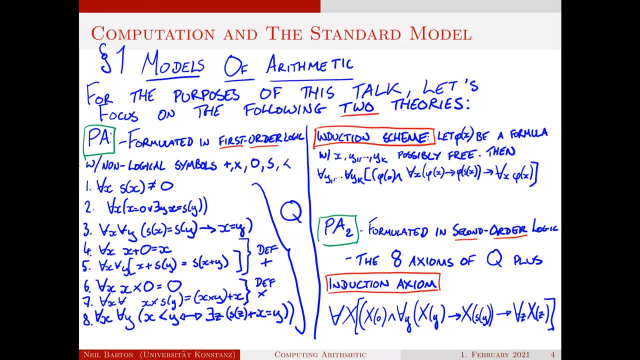 So we have just quantification into object position, and it has non-logical symbols. plus times nought successor less than You can also formulate this with a 1 instead of the successor, if you would rather. And then there are some fairly basic axioms. 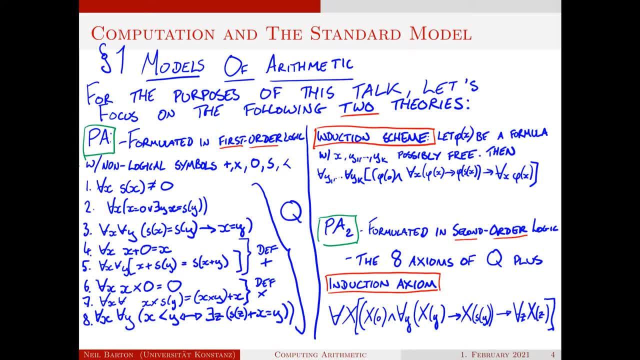 So we have firstly axioms for zero and how it behaves with respect to the successor operation, axioms about the successor operation itself, the recursive definition, the addition of plus and multiplication, and then an axiom about the less-than relation. And these eight axioms together form what's called Robinson arithmetic, or 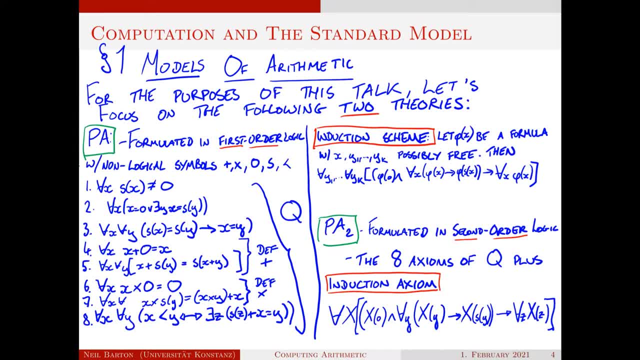 Q. Now the really important additional axiom to get you first-order piano arithmetic is the following induction scheme: Okay, so this says: look if I've got some formula phi right with a bunch of free variables, but importantly, x is one of these. 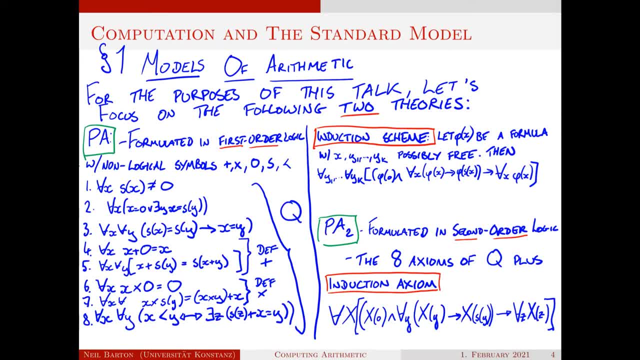 possible free variables, then if it holds zero and for any object, if it holds, then it holds at the successor of that number, then it holds for everything. Okay, so the sort of motivation for this is thinking of the numbers like dominoes, right? 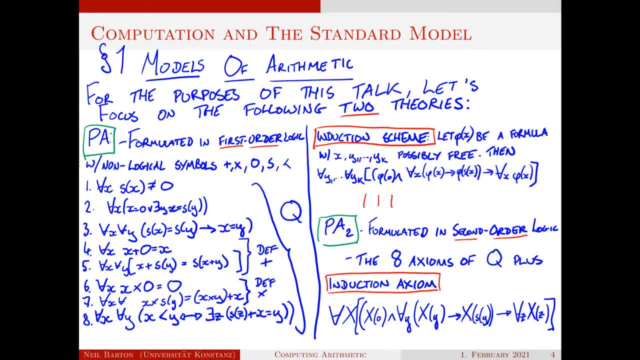 So I have zero and then I have one, and then I have two, and then I have three, and then I have four. Right, And I show that phi holds of zero, but I also show that if phi holds for any particular number, 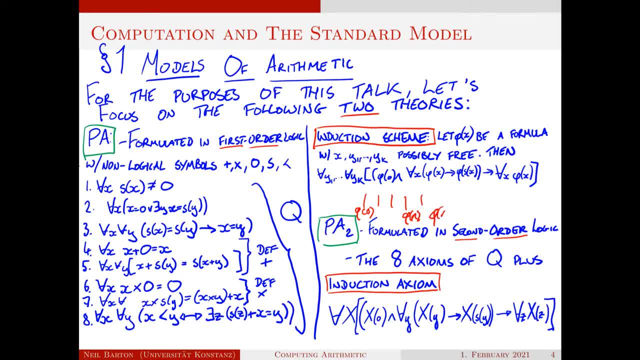 then it's gonna hold for the next number as well, right? And if I know that, then I know that phi doesn't just hold for zero, but because if it holds for any particular number, it holds for the successor. it's gonna hold of phi one, and 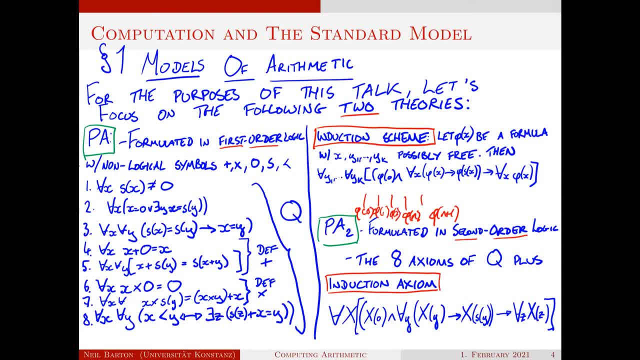 then we're gonna hold for phi two and so on. So it's the idea that we show that the first domino gets knocked over and then we show that if any domino next gets knocked over, then the next domino gets knocked over, right? 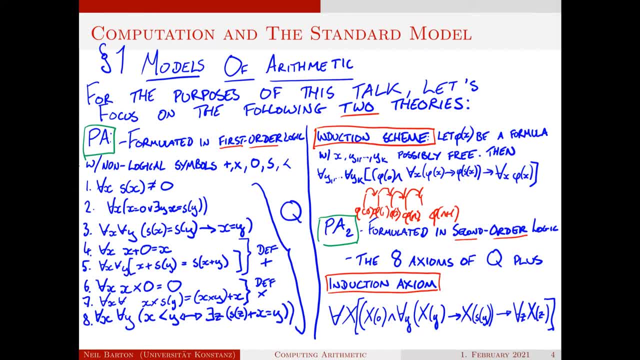 And so the motivation is that we thereby show it for all, all of the natural numbers. Good, A really significant point about the induction scheme is that it is exactly a scheme. So this is not one axiom, This is an axiom for every particular phi, in the language of arithmetic, of the required form. 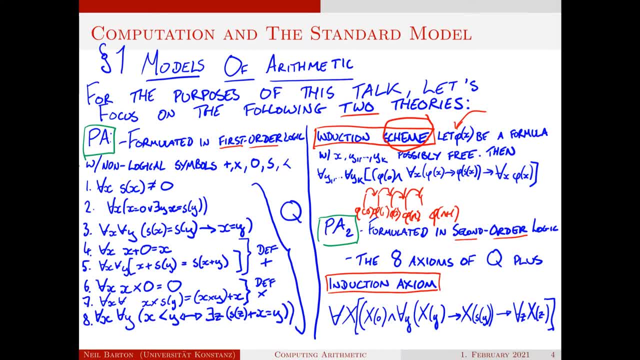 Okay, so Peano arithmetic. first order is not finitely axiomatized. It has infinitely many axioms, in particular one for each instance of the induction scheme. Now, this all changes when we move to second-order: Peano arithmetic. okay. 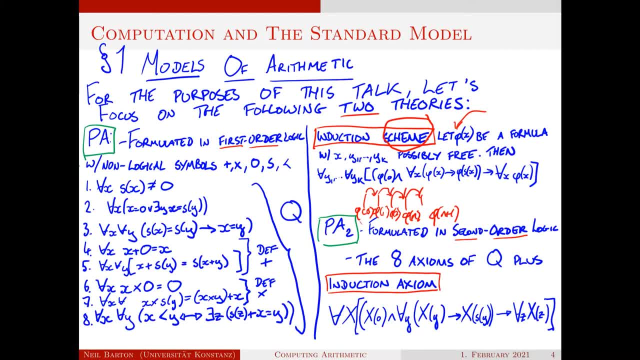 So second-order Peano arithmetic is formulated in second-order logic. This is where, in addition to quantification into object position right, we also allow quantification into predicate position right. So we can say things like there is a property y such that y holds of x, for instance, whereas that's not permitted in first-order logic. 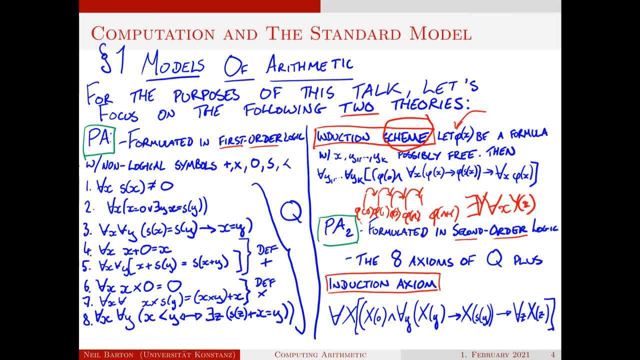 In this context we can formulate second-order Peano arithmetic, and this has axioms, the eight axioms of q. but instead of the induction scheme we've got an induction axiom where we say: for all properties, if they hold of nought and 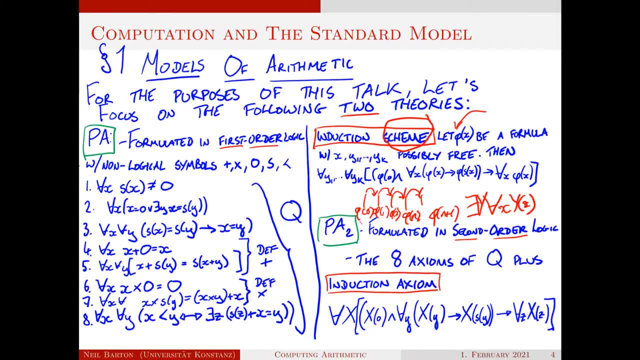 if they hold of a number, then they hold of the successor of that number. then that property holds for all numbers. okay, So we can replace this scheme in the second-order case with this axiom. Now this doesn't seem like a big difference, but once you come to look at the semantics for these differences, 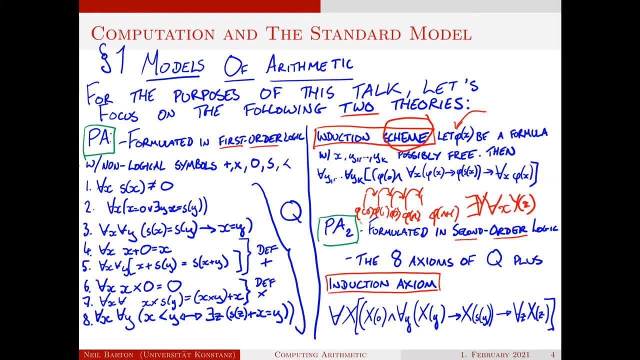 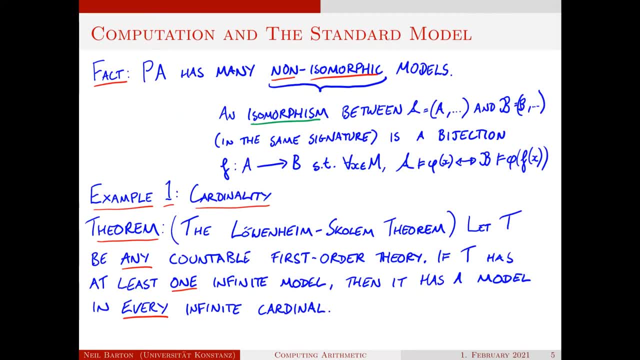 you can get some quite significant differences with respect to the kind of structure they can pin down, And we'll talk about that in just a second Good, so this, the worry we're going to look at- comes partially from looking at different models of Peano. 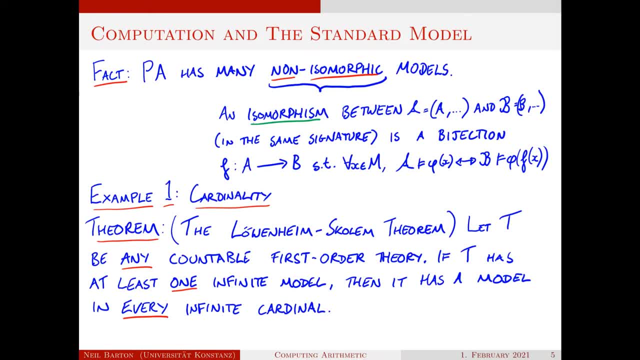 arithmetic, And a standard fact from out the model theoretic literature is that Peano arithmetic actually has the first-order version, has many isomorphic models. okay, What's an isomorphism? That's just a bijection between two structures, right. 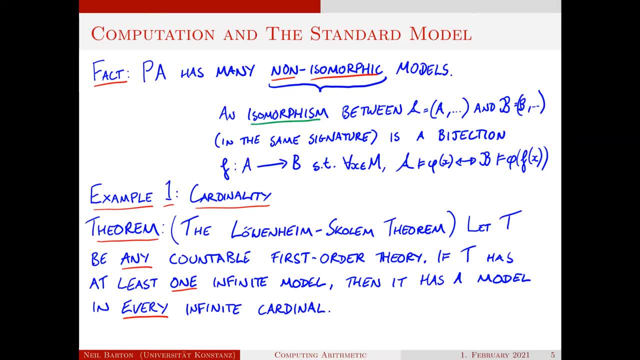 So this is a structure A, it has domain A and it has a bunch of relations and functions and so forth. and structure B has domain B and a bunch of relations and functions and so forth. As long as they're in the same signature, you can talk about an isomorphism in the sense that of a bijection between the two. 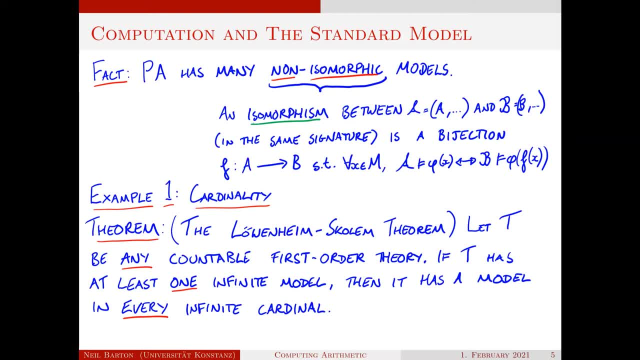 that preserves truth, right? So I have my structure A over here and I have my structure B over here, and an isomorphism is just a bijection between A and B, so it maps everything up one-to-one. But also when I look at any point A in A, 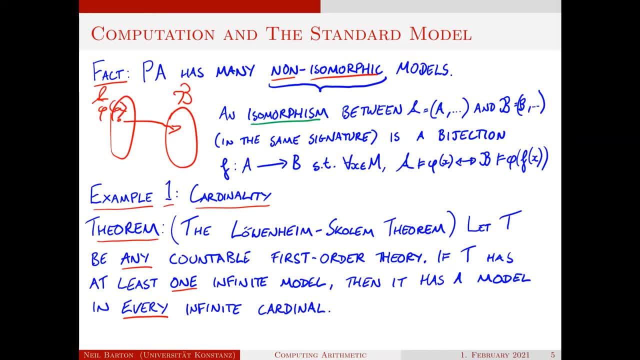 if phi A holds over here, I know that phi of F of A holds in B and vice versa. If I have some B here and phi of B holds here, then I know over here that phi of F- to the inverse of F of B- holds over here. 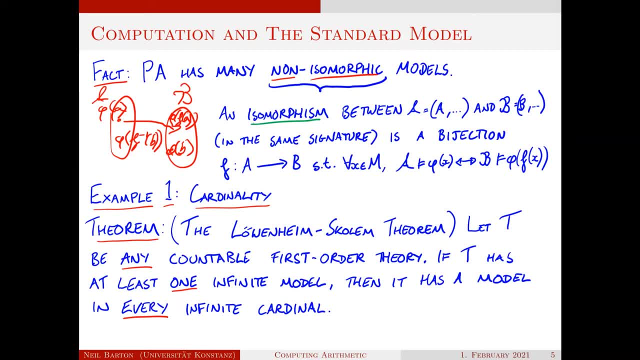 So it's one way of saying that A and B have the same structure. okay, I can pair them up in such a way that all the truth stays the same in the relevant language, no matter whether I go back or forth. Okay, and what we know from some model theoretic results is that this first-order theory of Piano Arithmetic, the kind of standard, 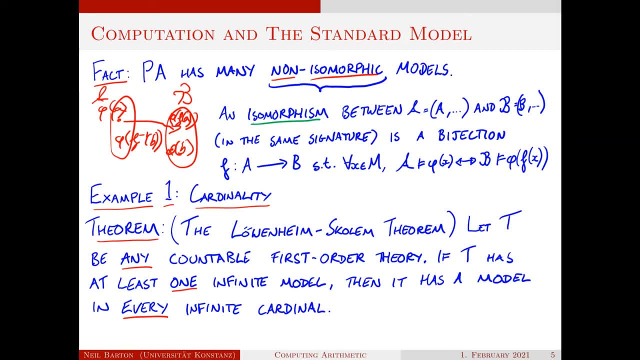 theory of the natural numbers we'd like to have first order has many, many non-isomorphic models, many, many models that differ on their structure. So here's one example, and to motivate it, we're going to look at the following theorem: 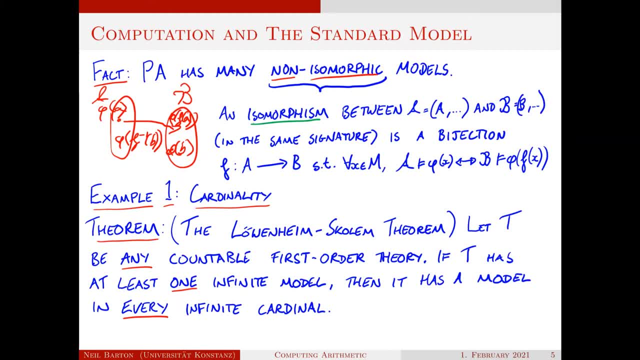 This is the Loewenheim-Scholem theorem and this states that if T is any countable first-order theory, if T has at least one infinite model, then it has a model in every infinite cardinal. So we talked a bit about in earlier weeks how there are many different cardinal sizes. right, I can have. 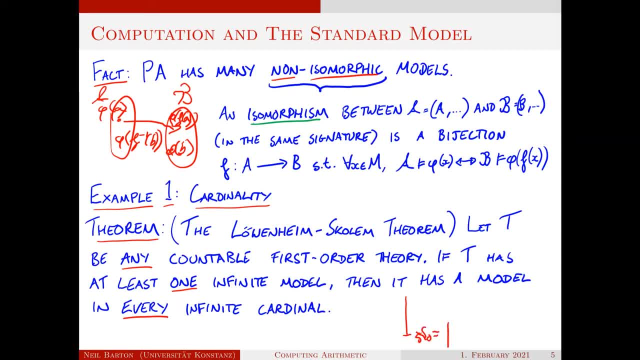 Aleph-naught. this is the cardinality of the natural numbers. this is the sort of smallest infinite cardinal, but there are many, many infinite cardinals. right, I can have Aleph-1, and so on, this huge hierarchy, And 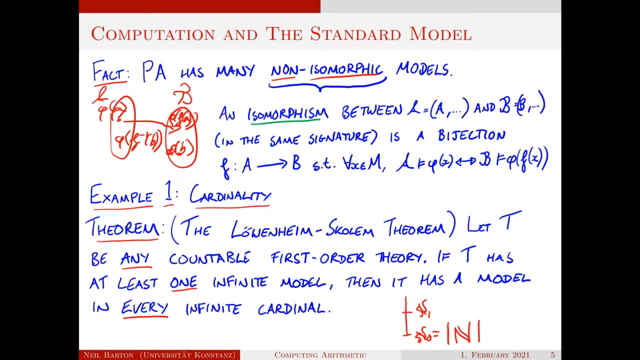 in particular. for instance, the cardinality of the real numbers is greater than the cardinality of the natural numbers. We don't know exactly where it fits into this Aleph structure. That's a difficult question in and of itself. It can be shown that you can't prove it from our standard set theory. but setting that aside, 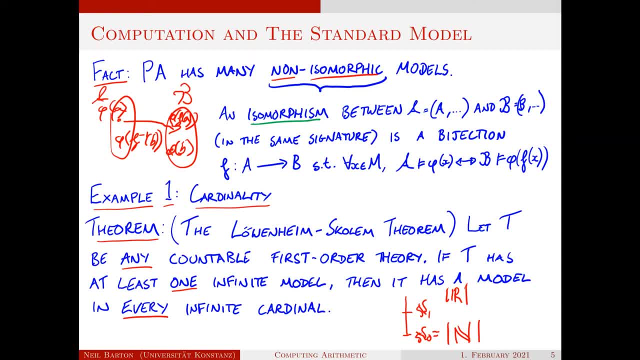 we do know it's bigger than the natural numbers. So we do know that there's this huge hierarchy of cardinals. Now what the Loewenheim-Scholem theorem shows you is that within this hierarchy, so long as my theory T has at least one model, 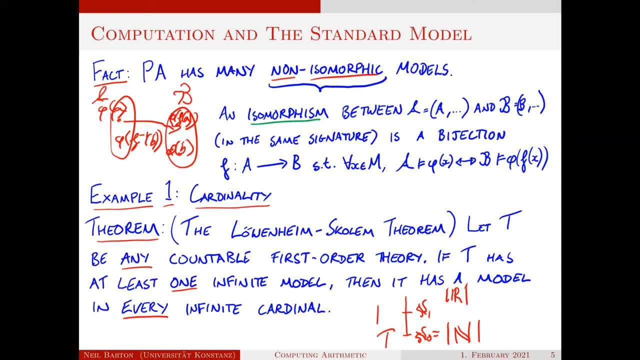 let's say, of size Aleph-naught. it's going to have a model in every larger infinite cardinal. So this in particular implies that you know you have countable models of Peano arithmetic. You'll have the standard model that we know and love. 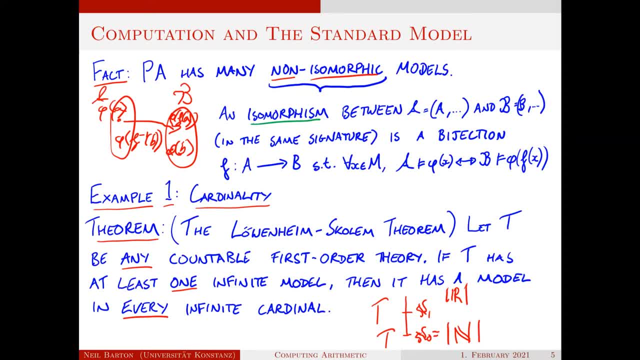 but there will also be lots of much, much bigger models and bigger cardinalities. So you have, for instance, a model of Peano arithmetic that's going to be the same size as the real numbers. for instance, There'll be some structure A that has the cardinality of the real numbers but is such that it models Peano arithmetic, for instance. 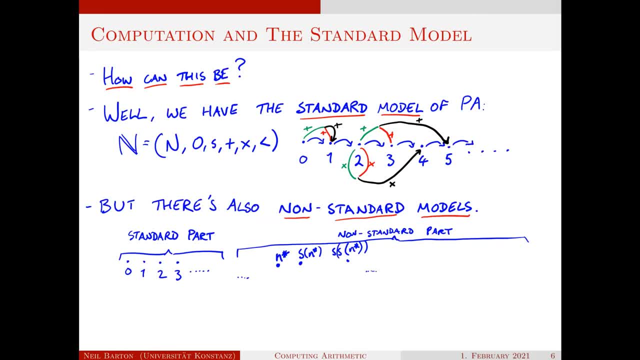 So an immediate question you might have is: how on earth can this be? I mean, I certainly was very confused by this as a beginning philosophy student, And the core point is that you can have models that have these so-called non-standard numbers. okay, So we're all familiar with what people often call the standard model of Peano arithmetic. 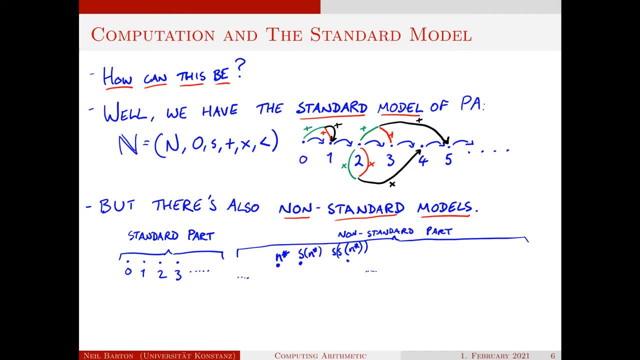 This is just your friendly number: 0,, 1,, 2,, 3,, 4,, 5, etc. And they have operations defined on the natural numbers, right. So we have the addition of 0 and 1, for instance, if we take: 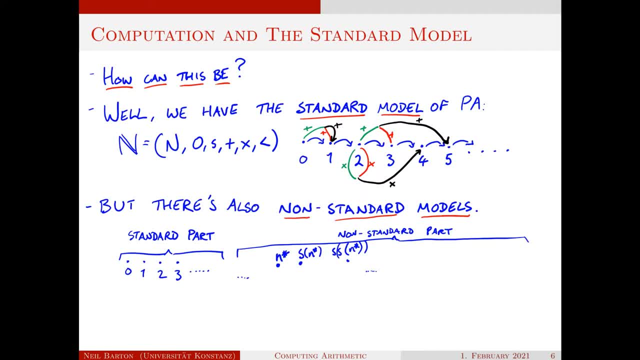 the green to be the first input to the function and the red to be the second. 0 plus 1 is going to give you 1, right. 2 plus 3 is going to give you 5, so on 2 times 2 gives you 4.. And 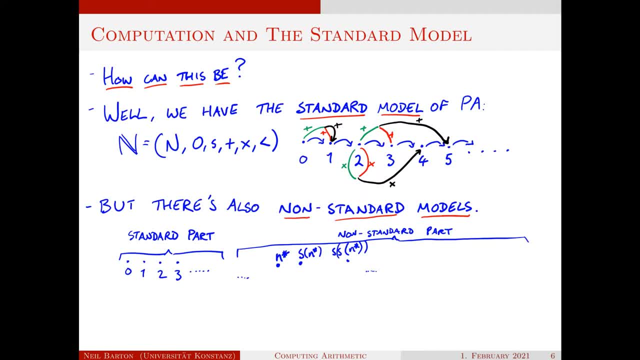 underneath it all, we've got the successor going along and, if we wanted to, we could talk about the less-than relation that goes backwards like this, for instance: right In the future, we're going to need a recursive model, and 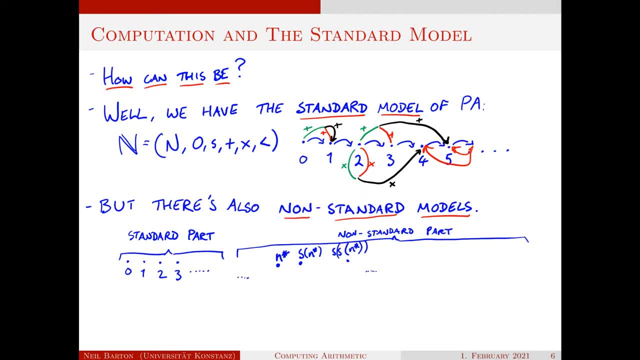 In addition to this friendly standard model, which is kind of what we normally think of the numbers as being, there are also non-standard models that satisfy Peano arithmetic. So we have the standard part, you know with the successor operation going off, but we also have 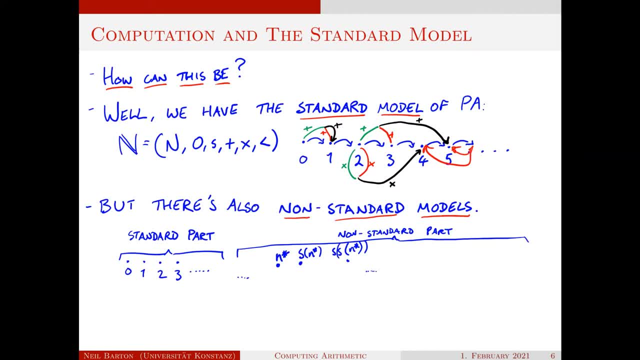 these weird infinite natural numbers in inverted commas, what the model thinks are natural numbers beyond all the natural numbers we normally think of. Peano arithmetic itself can't fix the standard model. You can also have these odd non-standard model numbers off past the standard numbers you'd. 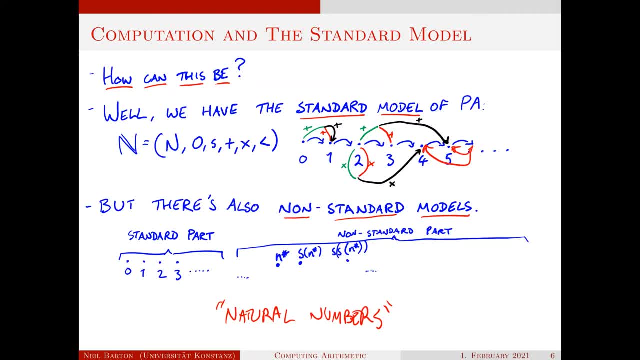 consider, And the operations will also be defined on these non-standard natural numbers as well. So, for instance, the successor operation still holds there, because you know it's one of the axioms of Peano arithmetic that every natural number has a successor. Okay, Now this is where we can bump up the cardinality very high, right. 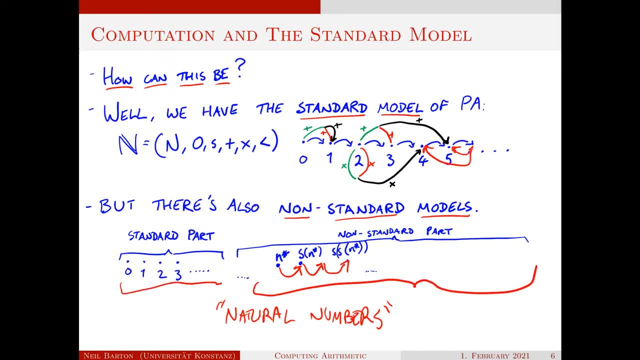 As in the Lohenheim-Skodum theorem, this part is always going to have cardinality aleph-nord, but we can perfectly well stick in kappa many natural numbers or inverted things that the model thinks are natural numbers For any particular kappa that we pick. 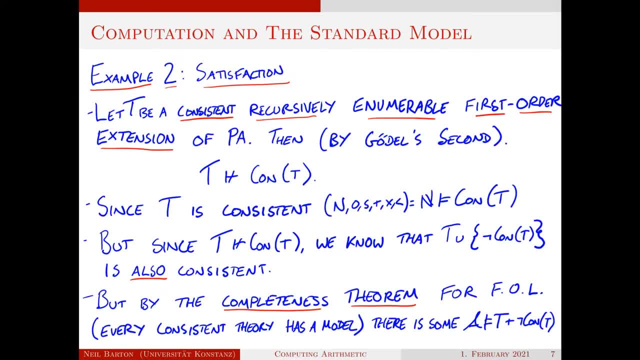 Another place we see non-standard models crop up is with respect to the sentences satisfied by the relevant models. So in the last case we looked at, we were bumping up the cardinality of the model quite significantly. But you can also have models that are countable but satisfy different sentences. 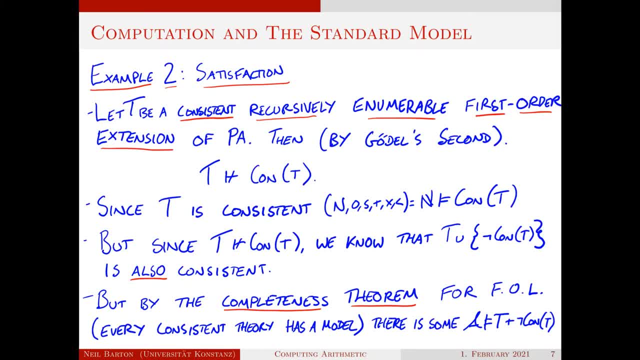 from each other. So this is a really good example of a non-standard model. So a neat example for seeing this is with respect to consistency sentences. Now, we discussed consistency sentences a little bit earlier in the context of Gödel's incompleteness theorems. 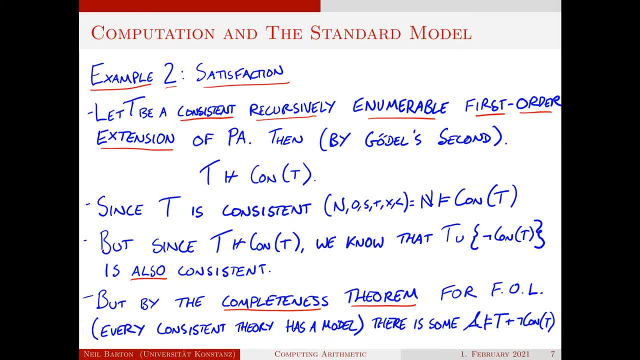 Okay, Now let's just recall a little bit of the details there. So if we let T be a consistent, recursively enumerable first order extension of first order Peano arithmetic, then we know by Gödel second incompleteness theorem that T does not prove its own consistency sentence. 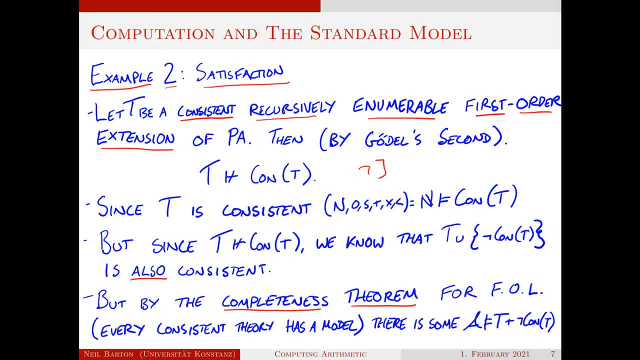 Recalling that the consistency sentence says that it's not the case that there is some x such that x codes in T a proof of zero equal one. right Now, since we're assuming that this particular T is consistent, we know that the real natural numbers satisfy con t. So there is no proof of 0 equals 1 in t by assumption. 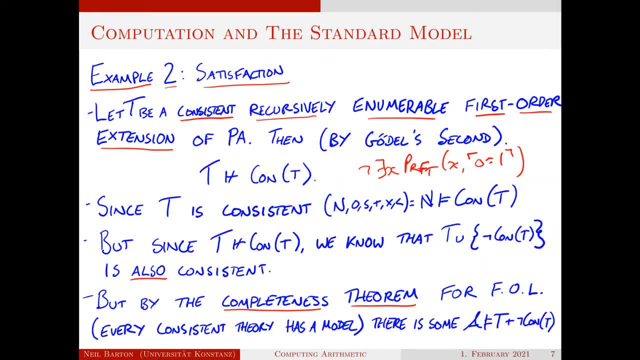 and so on, the natural numbers. when we look at codes of proofs, there's going to be no such proof and so they're going to satisfy con t. But we also know that, since t does not imply proof, theoretically speaking con t, we know that t with con t, with the negation of con t added to it, is also consistent. 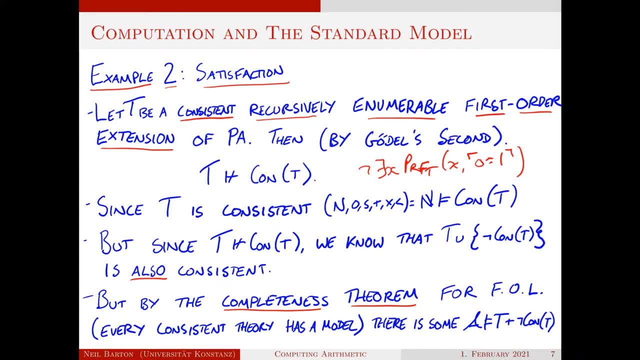 okay, something doesn't, for first order theory does not prove a sentence. I can add that that sentence to the theory. consistently Okay, but now this critter here. this is a consistent theory and so we know by the completeness theorem for first order logic, the theorem that every consistent theory has a model, that there is some model satisfying this. 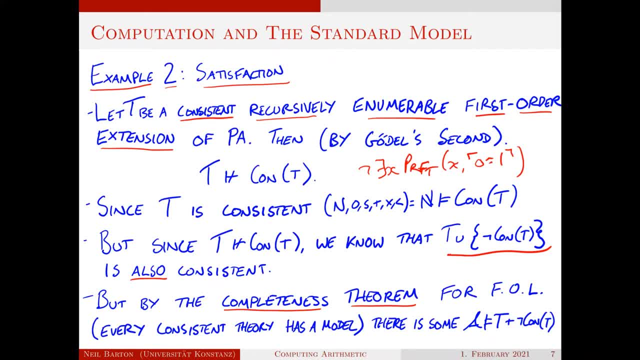 theory t plus neg con t or not con t. Okay, but this is a really baffling thing, right? this model a both satisfies the theory in question, but also thinks that it's inconsistent. So what on earth is going on here? Well, here's what's going on. 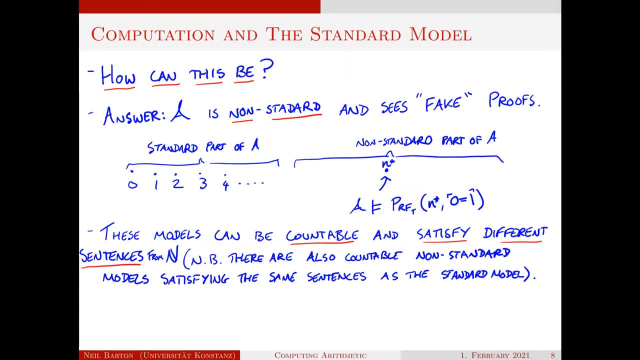 In this context, our structure A, satisfying t plus, not con t. so this is our structure A and let's remember that it satisfies t plus, not con t. A is very confused about what the natural numbers are. There are crazy things it thinks are natural numbers that are not real natural numbers. Now, remembering the natural numbers: code up proof. 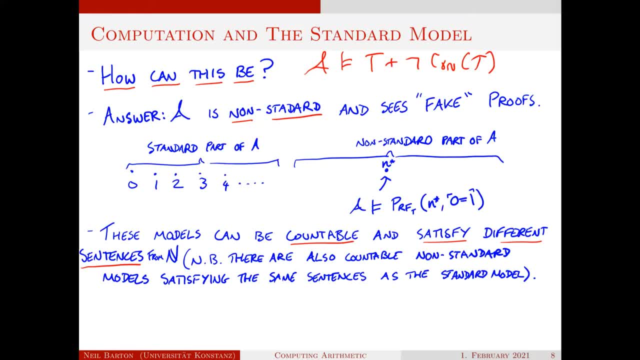 right. what's happening is that our structure A is seeing some fake proofs, seeing some not real proofs in the non-standard part of A right. so on the standard part of A, it's not the case that not con t appears here, but there's some wacky, non-standard natural number. that is that A thinks. 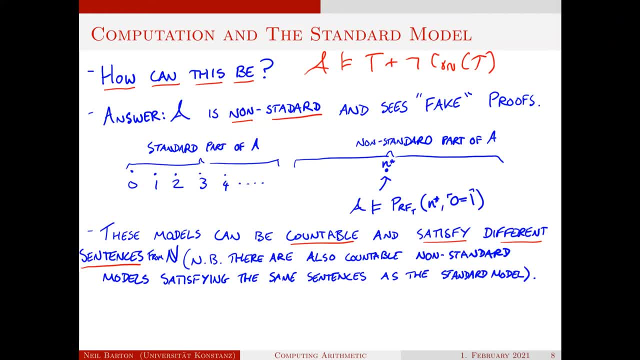 codes a proof of zero equal one in t. This is not a real proof. this is some crazy infinitary object that A cannot distinguish from the regular natural numbers. it thinks it's a natural number, but it, according to A, codes a proof of zero equal one in t, right? So this is what's going on here and these things can. 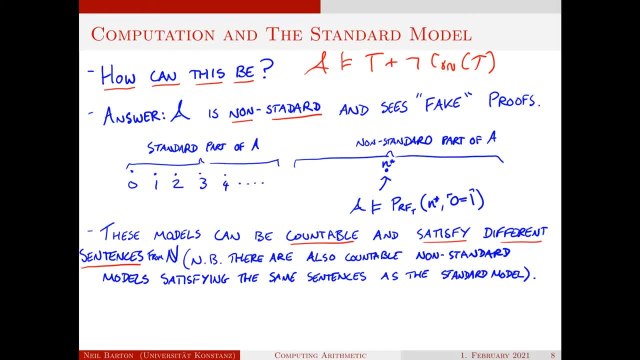 perfectly well be countable, right, and they satisfy different sentences from the standard natural numbers. So what you have here is you have a particular model of arithmetic that is potentially countable but also is very confused about what the sequences are right. It's confused about what the proofs are. 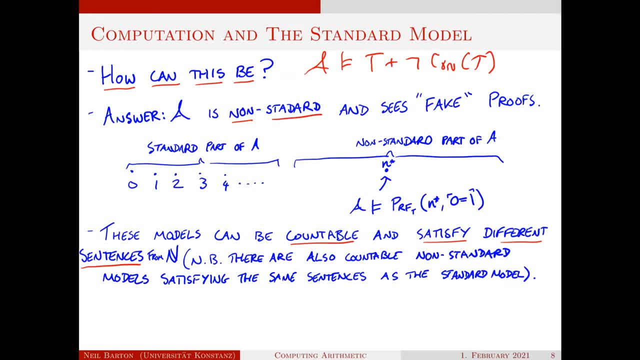 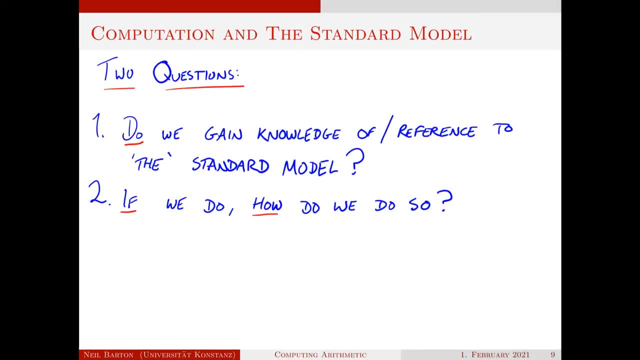 and for that reason it thinks that, uh, thinks that sentences are well sorry, theories are inconsistent, that are not actually inconsistent. Okay, So We have these two model, theoretic, uh kinds of observations that show that first-order piana arithmetic does not pin down the, uh, the standard model of arithmetic for us. 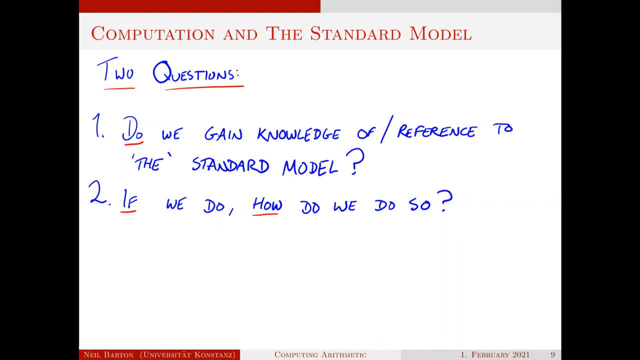 Now there's a sort of skeptical position you might adopt on the basis of these two. so if it's not the case that you know our usual theory of arithmetic, piana, arithmetic pins down the standard model for us- you might worry that actually thought and knowledge is not determinate about the standard model. rather, we are only able to. 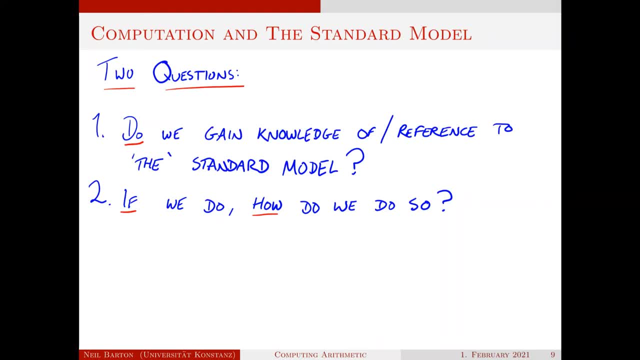 talk kind of schematically about, uh, different models of first-order piano arithmetic, and our thought and language doesn't suffice to pin down the standard model. okay, so there's kind of two. we have this skeptical worry And uh, with this skeptical worry, we have kind of two questions or challenges, and the first is that 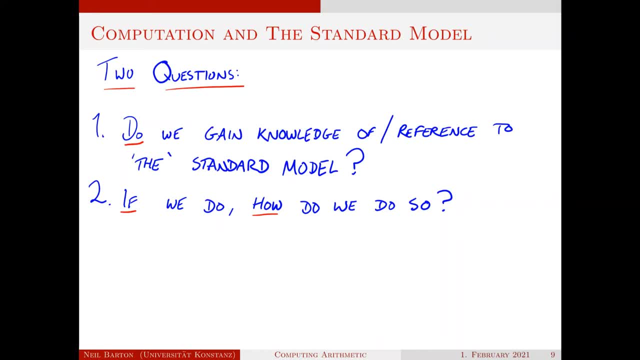 well, is the skeptical worry true? do we gain knowledge of or reference to the standard natural uh, the standard nat model of the natural numbers, or are there rather uh just schematic talk about many uh models of first-order piano arithmetic? and indeed, if we are able to gain knowledge of reference? 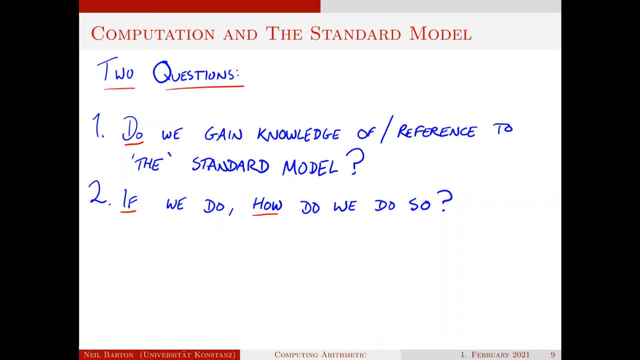 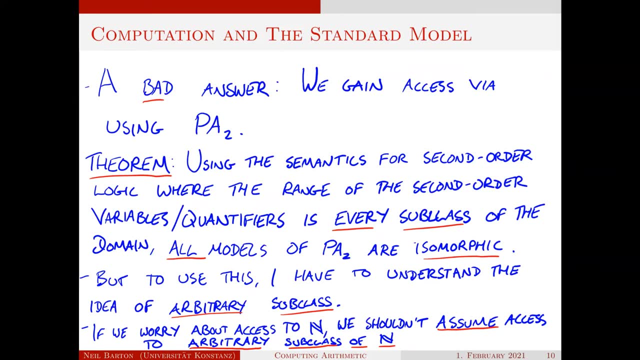 to the standard model of natural numbers. how do we do so, or perhaps how can we do so? Now, there's an immediately uh kind of bad answer we could give to this skeptical challenge, and that is that we gain access, uh via using second-order piano arithmetic. 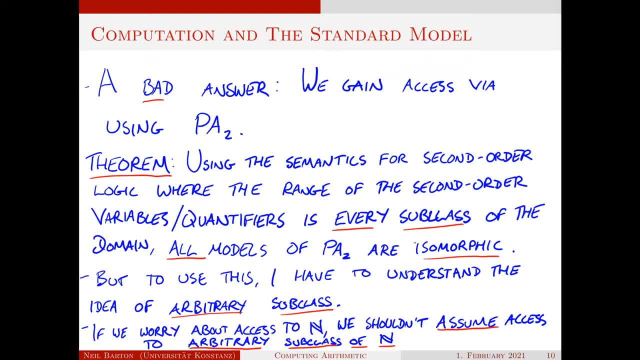 We might point to the following following theorem here, and that's using the semantics for second-order logic, where the range of the second-order variables or quantifiers is every subclass of the domain right. All models of second-order piano arithmetic are isomorphic, so as long as we 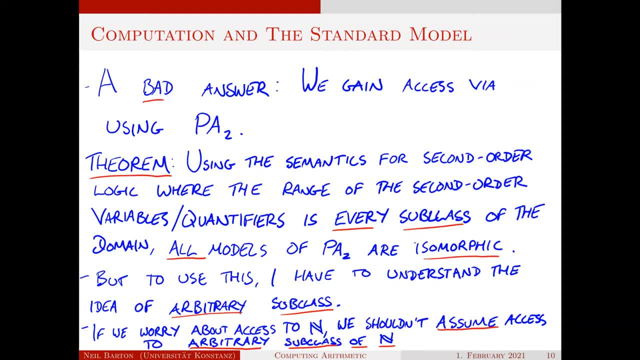 have access to all the subclasses of the domain. uh, I can show you that if that thing satisfies second-order piano arithmetic, it's isomorphic to any other thing. Uh, satisfying second-order piano arithmetic with the um, with the full subclass, uh interpretation, okay. so in the context of second-order piano arithmetic, as long as we have a very strong 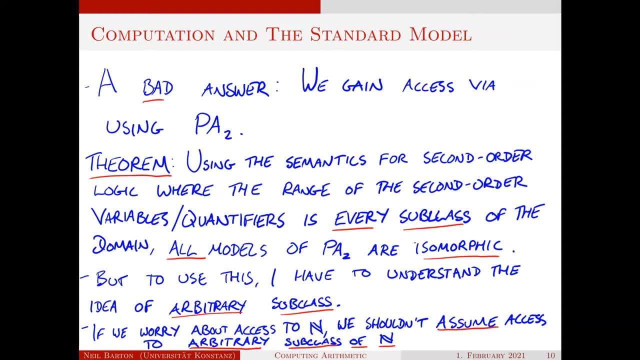 kind of semantics in the background. we do get uh characterization up to isomorphism okay, but there's a kind of uh. although this is a perfectly good um result from model theory, it's kind of unsatisfying in the context of responding to the uh challenge of the skeptic because in this case I have to use the idea of an arbitrary. 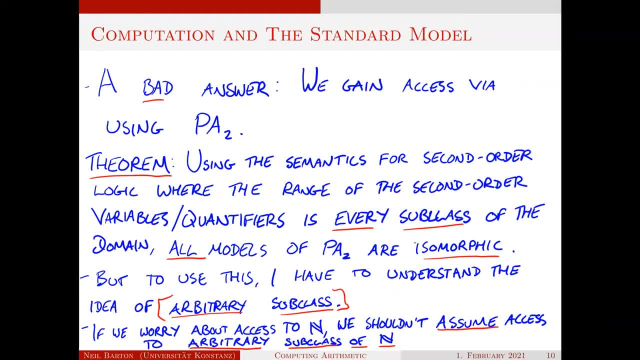 subclass of natural numbers in making it precise what the natural numbers are. so if I'm already worried about what my access to the natural numbers might be, it's no good for me to assume access to arbitrary numbers. haha, it's not ideal, which, I guess, is why natural numbers really exist. 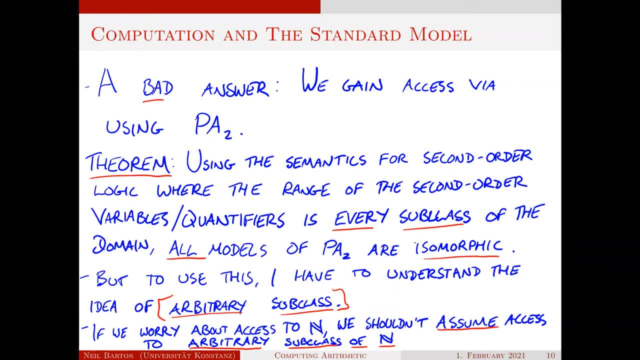 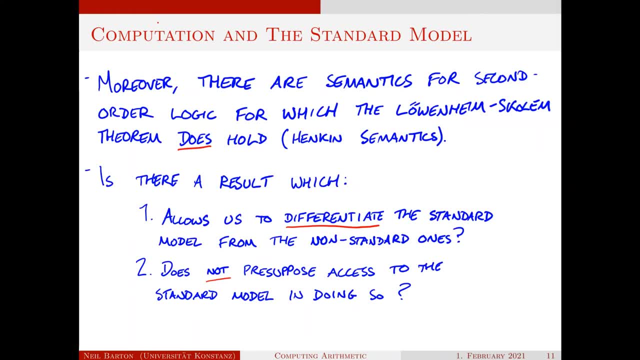 the notion of arbitrary subclass of natural numbers. This issue is made even more acute when you look into the model theory a bit and you can find these semantics for second order logic. These are called Henkin semantics, for which things like the Lowenheim-Scolan theorem does hold, And in fact 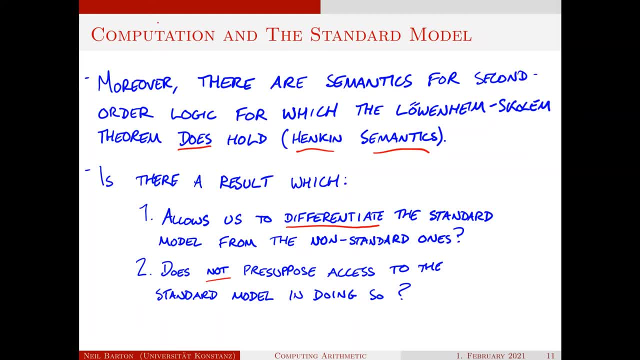 in this context, second order theories are equivalent to two sorted first order theories in the kind of properties they have for Henkin semantics. So they have, if you know, some model theory. they have things like compactness properties and they have, as I said, the Lowenheim-Scolan results hold. 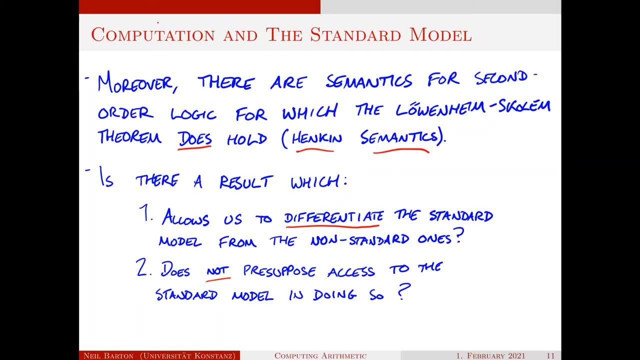 So the point is that this requirement that I have the full notion of arbitrary subclass in the background is important for getting this and indeed essential for getting this characterization of the natural numbers up to isomorphism within second order piano arithmetic. But this kind of 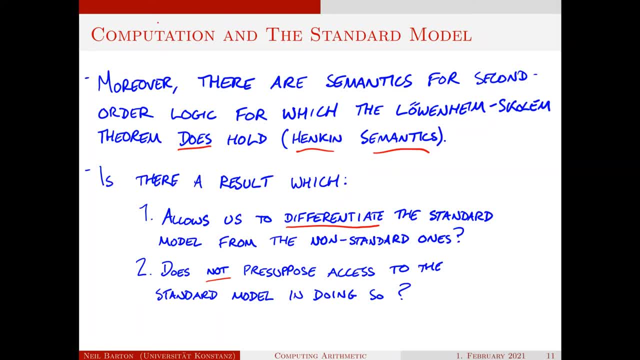 observation. this kind of response does raise the following possibility or suggestion, and that is: look, is there a rational formula, Is there some sort of result that we can appeal to from model theory or our understanding of natural numbers that, firstly, allows us to differentiate the standard? 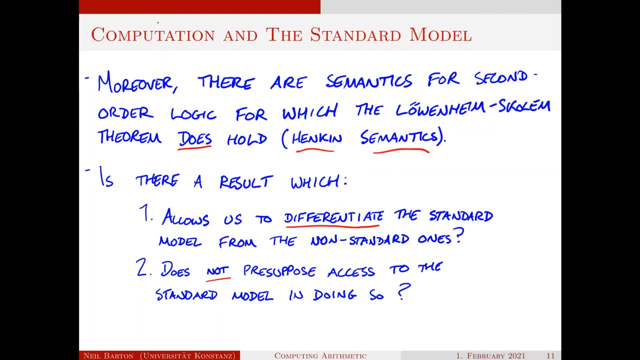 model of arithmetic from the nonstandard ones, but does not presuppose access to the standard model. in doing so, Or in the case of PA2, something it seems even stronger than the standard model, the idea of arbitrary subclass of natural numbers. And this is exactly where results about computability are going to come in. 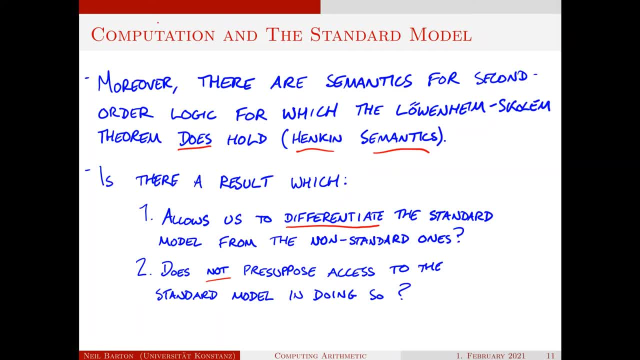 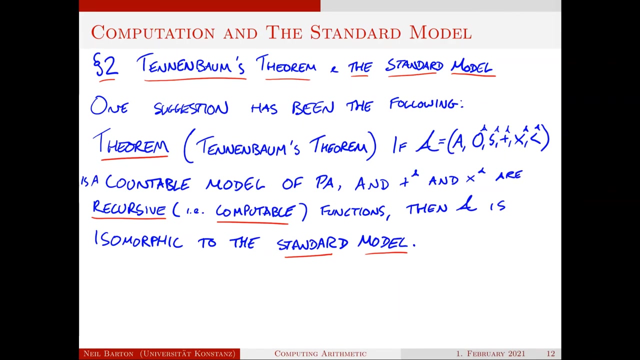 The idea is going to be that look, the non-standard models do not obey principles we think the natural numbers should have with respect to the computability of the multiplication and addition operation. So one suggestion that has been made several places in the literature is the idea that the following theorem, called Tenenbaum's theorem, does the job for us. 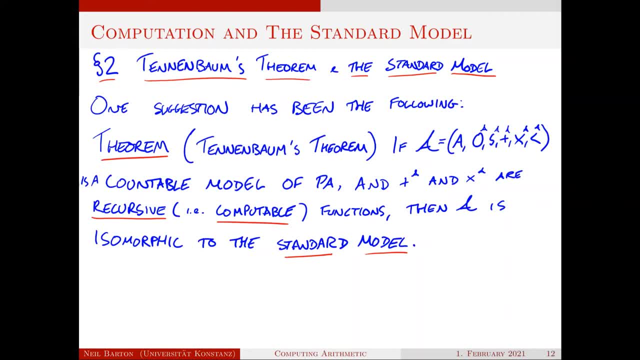 So Tenenbaum's theorem is the following: So it says that if some structure A which has domain A has an interpretation of zero successor, plus times and less than is a countable model of Peano arithmetic, and plus and times are recursive, ie computable functions, then A is in fact isomorphic to the standard model of arithmetic. 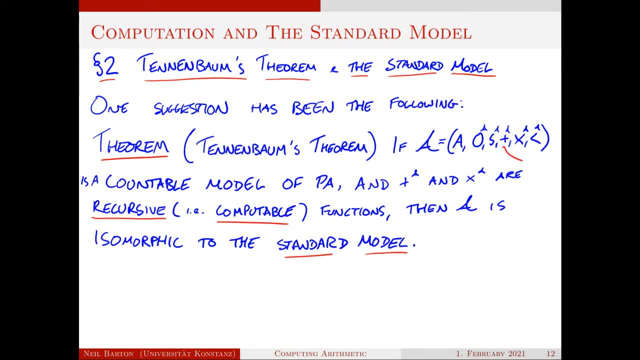 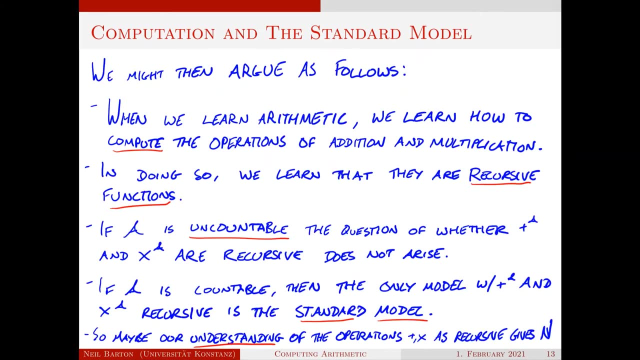 So the only times where we can have plus and times to be computable are exactly in the case in which A is isomorphic to the standard model of arithmetic. Okay, with this in hand, we can run the following kind of philosophical argument: 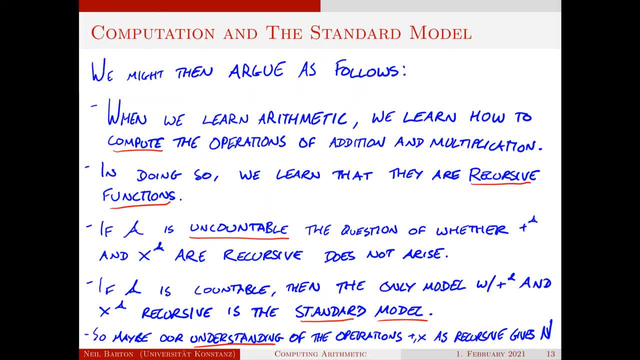 We might say that, look, when we learn arithmetic, we learn how to compute the operations of addition and multiplication. This is the kind of thing we do at school: We learn how addition and multiplication behave And as part of this we learn the particular recursive rules for addition and multiplication and we kind of see that they're going to be computable. 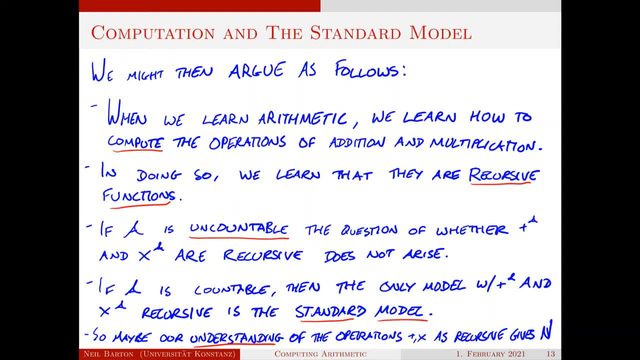 Right And you know, in doing this, we see that they're recursive, We see that they're computable, We have the rules for how they should be applied And we can see that whenever we get two numbers, there's a way of computing their sum or their product. 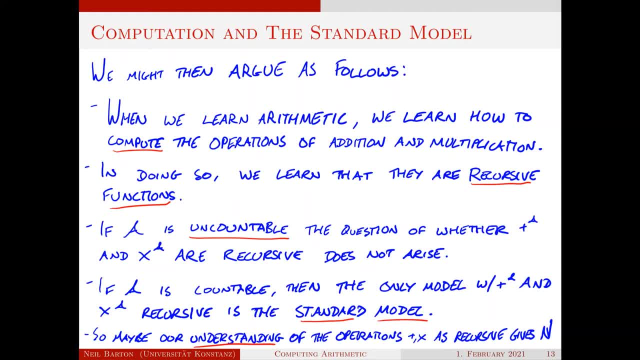 Right Now, if A is uncountable, this is our possible structure of the natural numbers. The question of whether plus and times are recursive does not arise. You can't have computable functions if the domain in question is uncountable. 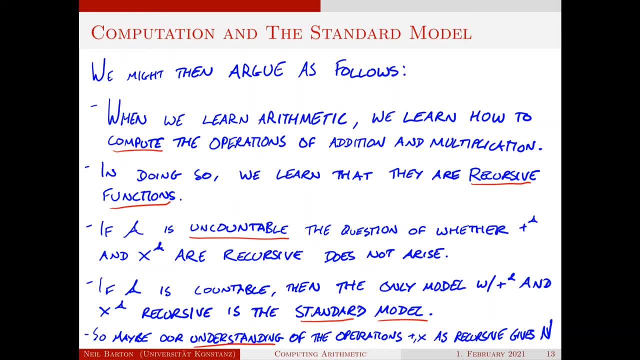 It's just too many things. You'll never get to the uncountable entities. Okay, But if our model is countable, then the only model we have with plus and times recursive by Tenon-Bounds theorem is the is the standard model. 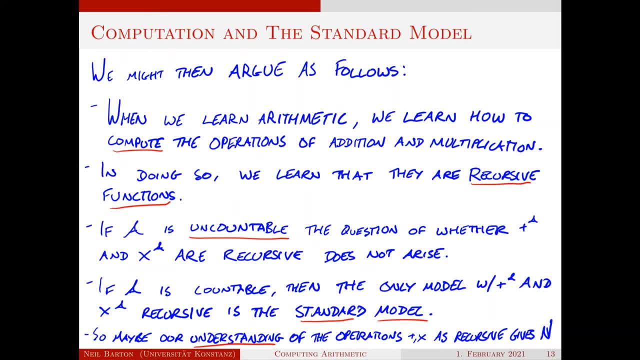 So the argument goes: look, we understand that the operations plus and times must be computable, And this perhaps gives us access to the standard model of arithmetic. Knowing that plus and times are computable, we then know that that thought and language refers only to the standard model. 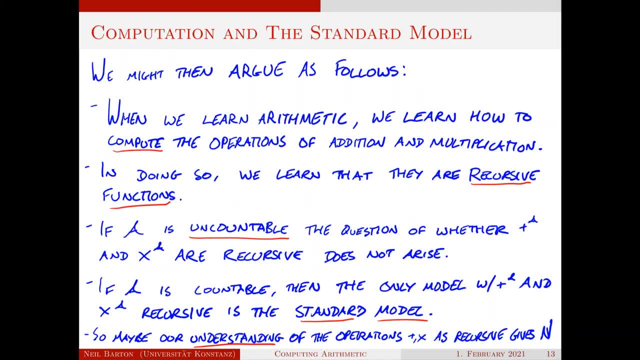 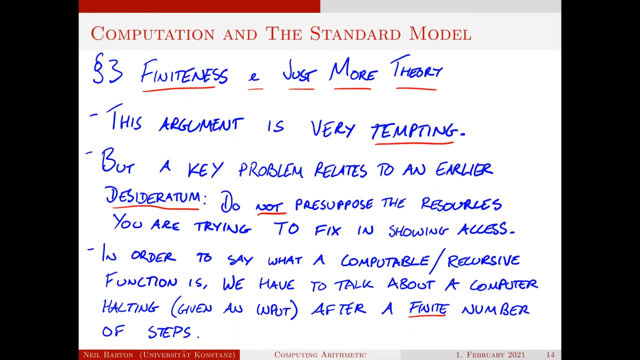 Of arithmetic when we want it to, Because for the other models they have non-recursive addition and multiplication operations. Now, on the one hand, I think this kind of argument is very tempting And I think Tenon-Bounds theorem definitely has philosophical implications. 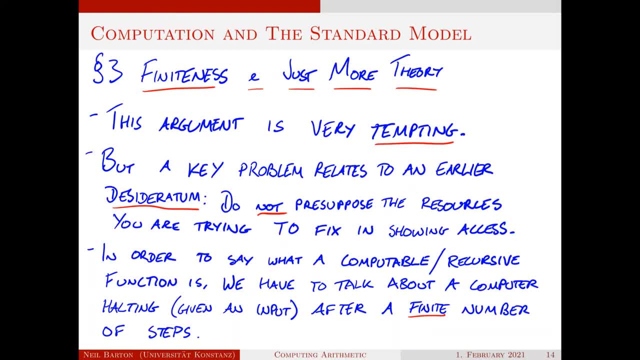 But I also think it should be unconvincing to the, to the, to the, the model theoretic skeptic. And this is dealt with very nicely in a paper by Button and Smith called the Philosophical Significance of Tenon-Bounds Theorem. 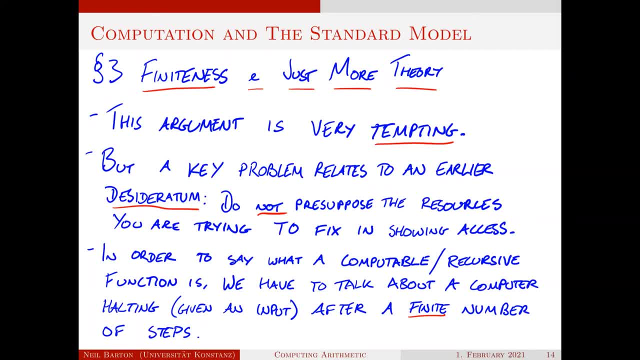 And the key problem is this earlier desideratum that we, that we looked at, that you should not presuppose the resources you are trying to fix in showing access. So, in particular, we can't presuppose access to the natural numbers in trying to show. 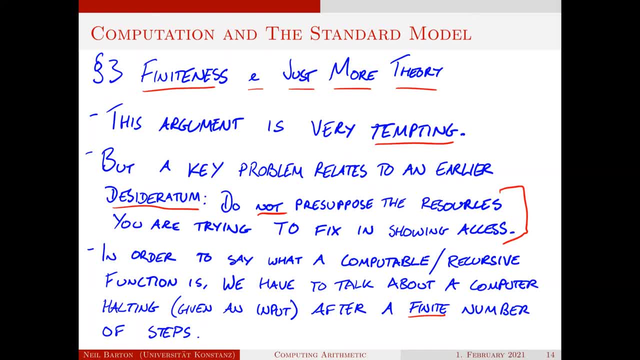 that we have access to the natural numbers using some model theoretic results. if we want to answer the skeptic right- And this is in particular only for answering this kind of very strong model theoretic or natural number skeptic- I'll say a little bit about what the place of Tenon-Bounds Theorem might be, if you're not a skeptic in the conclusions. 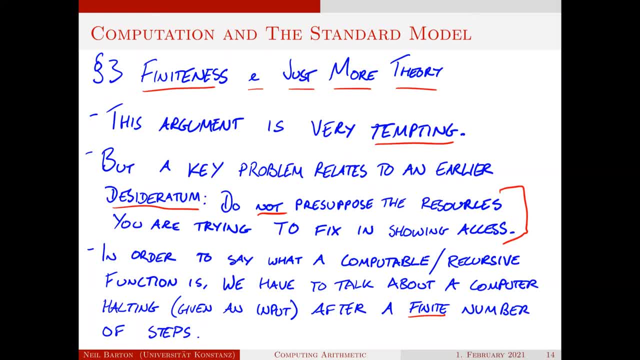 And the core problem is that in order to say what a computable or recursive function is, you have to talk about a computer halting or some equivalent in terms of recursiveness, given an input after a finite number of steps right, I have to appeal to the notion of finiteness in characterizing what it is for a particular function to be computable or recursive. 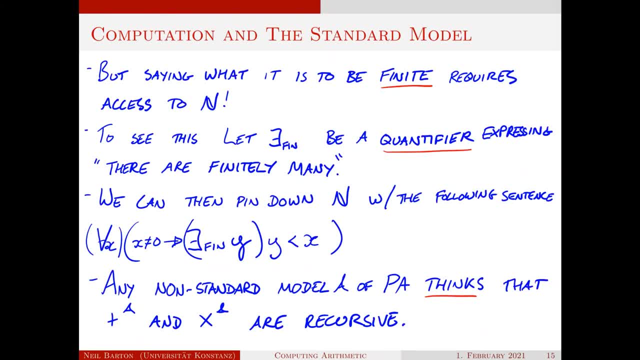 So let's look at this. We can see how deeply this kind of runs, Saying what it is to be finite, really does require access to the natural numbers. And to see this, let's introduce the following quantifier into our language: Let's have there exists thin to be a quantifier expressing the claim that there are finitely many right. 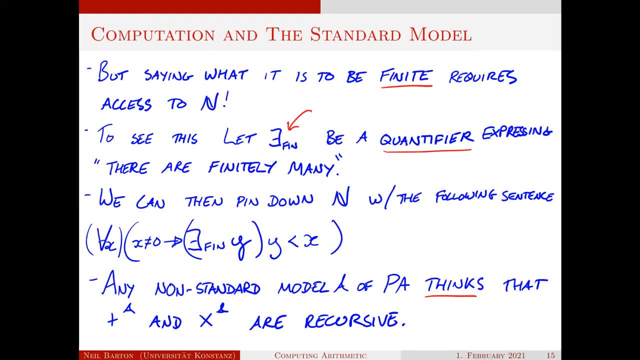 Now assume we give this quantifier a number And if we simplify its sort of standard interpretation, you could then pin down the natural numbers with the following sentence: right, You say that for any x, if x is not equal to 0, then x has exactly finitely many predecessors. 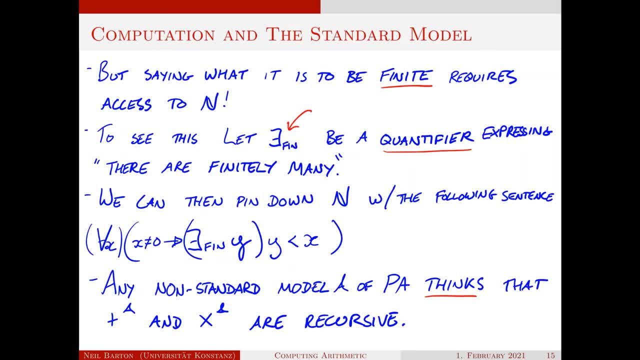 So it has finitely many predecessors, right? So the thought is here I have some model of arithmetic And for all I know it's nonstandard. But if I say that for any particular member of this structure there's only finitely many predecessors, then I'll be able to distinguish it from the nonstandard models. 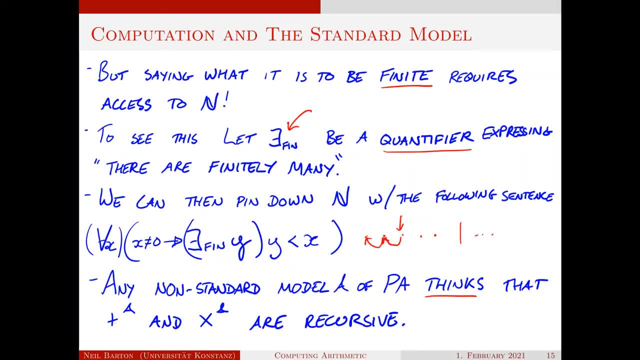 Because the nonstandard models have all these wacky nonstandard numbers out here which have infinitely many predecessors. okay, In particular, the whole standard part is going to. each member of the standard part is going to be a predecessor of this structure. 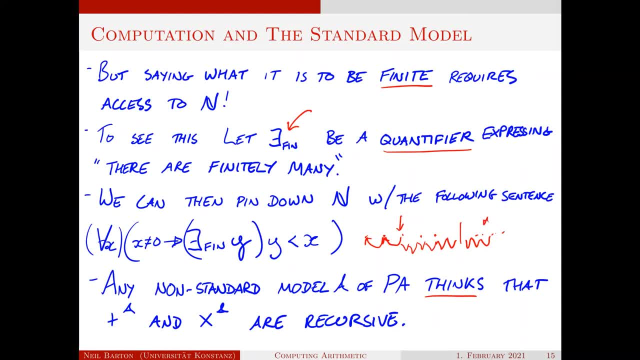 Okay. So we're going to be able to distinguish this of some n star in our wacky nonstandard model. So if you introduce any notion of finiteness and say it's determinately understood, it's going to allow you to pin down the standard model of arithmetic anyway. 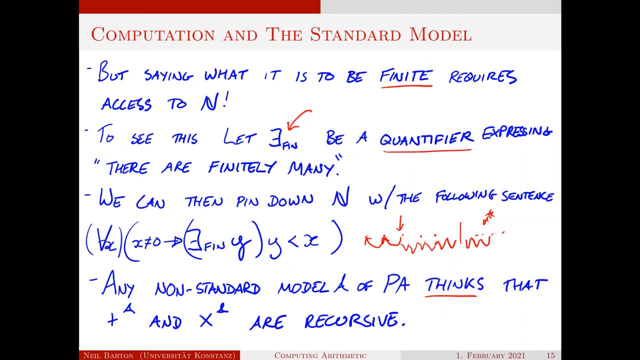 And in some sense, pinning down finiteness is just assuming access to this idea And in some sense, pinning down finiteness is just assuming access to this idea. And I think this is more vivid when we consider that, for instance, any nonstandard model of PA will think that it has plus and times recursive right. 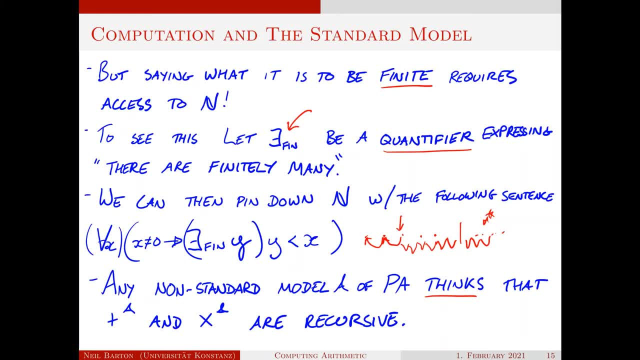 And I think this is more vivid when we consider that, for instance, any nonstandard model of PA will think that it has plus and times recursive right. So our particular wacky model here: right, it thinks that the operation of plus and times is recursive, even though it's not. 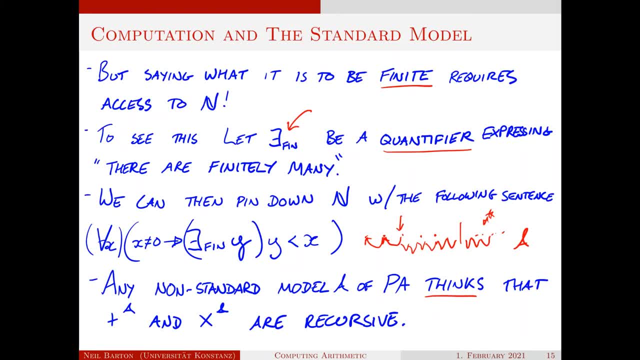 Why is this the case? Well, it's very similar to the cases to the Gauss-Hallis. Well, it's very similar to the cases to the Gauss-Hallis case. it's very confused about what numbers are really finite, right? so it might think that this 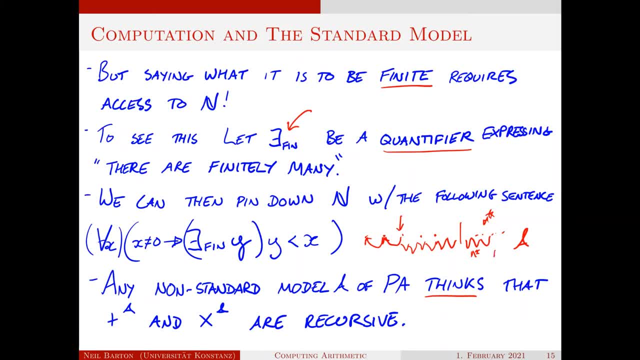 you know n star plus some other n star. let's call this n star naught and this n star one. it thinks that this operation here is recursive, but it only does that because it can do you know large, infinitary kind of computations. it's confused about what is really a finite computation. 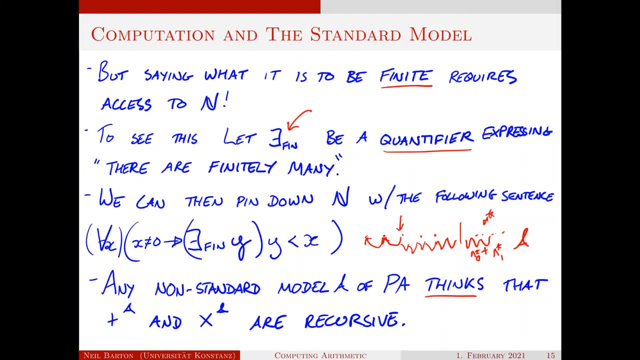 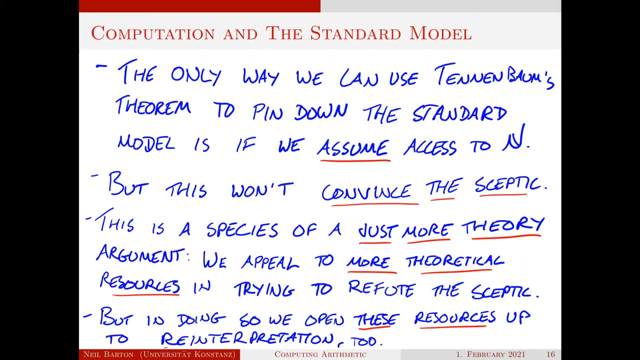 right. it's only when we step outside the model using our understanding of natural numbers that we see that a was confused about what the recursive functions are. okay, so the only way we can use tenon bounds theorem to pin down standard model is if we assume access to the natural numbers in 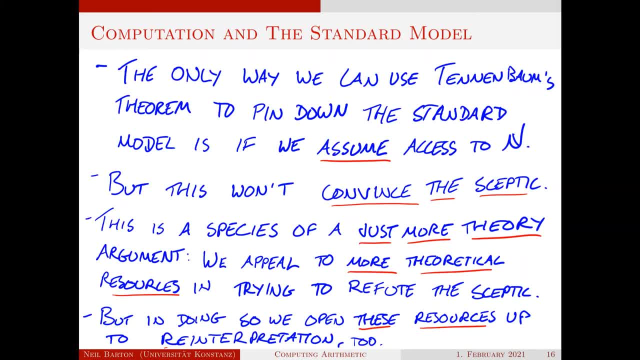 characterized in the notion of computation. and this isn't going to convince the uh, the skeptic about the natural numbers, precisely because they're not going to think that we have uh, or they're worried about our access to the notion of finiteness anyway. so this is, uh, an interesting 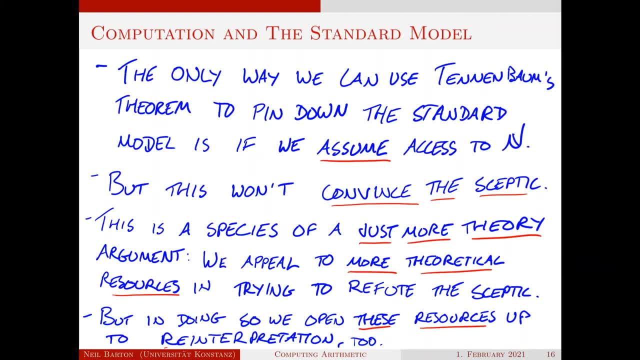 uh kind of argument, because it's a species of what's known as a just more theory argument. okay, so these are arguments. they appear a lot in uh philosophy, in the philosophy of language, in the philosophy of mind, where we have some kind of skeptical worry about reference or indeterminacy and we appeal to more theoretical resources in 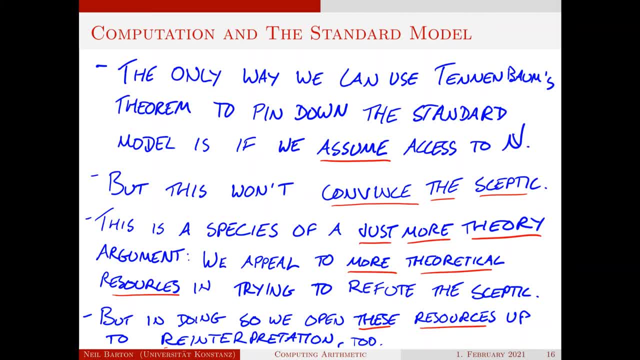 trying to refute the skeptic. so one example, for instance, is, if you're worried about the reference of our properties in general, you might move to talking about natural properties. there are only properties that, uh, carve at the joints. those are the only legitimate properties. so we're just gonna try and get that right here. so we're just going to have a a step. 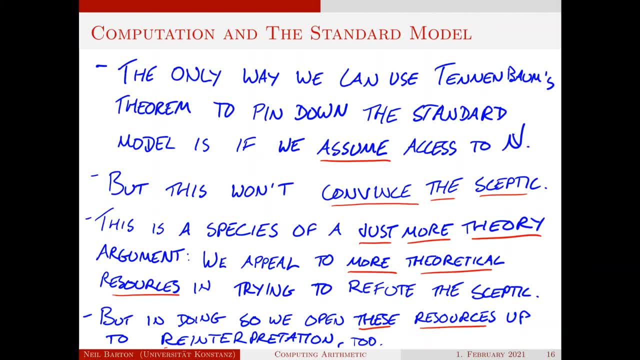 properties, something along that lines, those lines. The problem is with these kinds of responses in general across philosophy, is that when you appeal to just more theory, you open this extra theory you've appealed to up to reinterpretation too, right? So this is exactly what happened in this context. 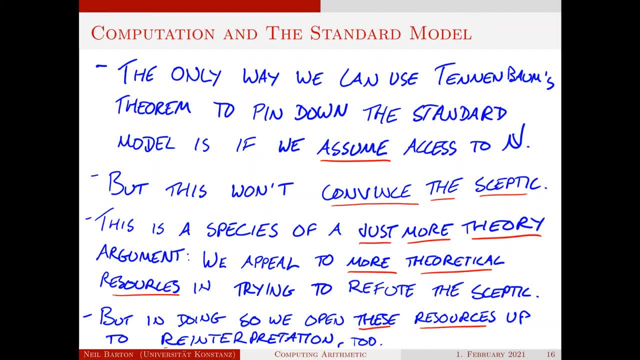 We appealed to a notion of computation, but that in turn is open to reinterpretation. if you don't or you aren't sure that we have standard access to the natural numbers. Similarly, if you think there are natural properties, you might think that the idea 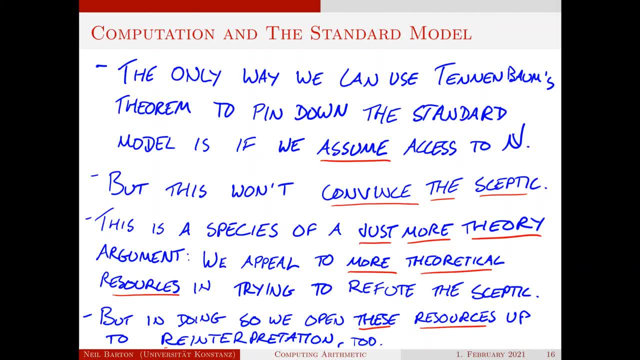 of a natural property is up to reinterpretation. This is dealt with in a lot of detail In Tim Button and Sean Walsh's book Philosophy and Model Theory, if people want to look at that more. The core point here is just that if you are going to appeal to a just more theory type, 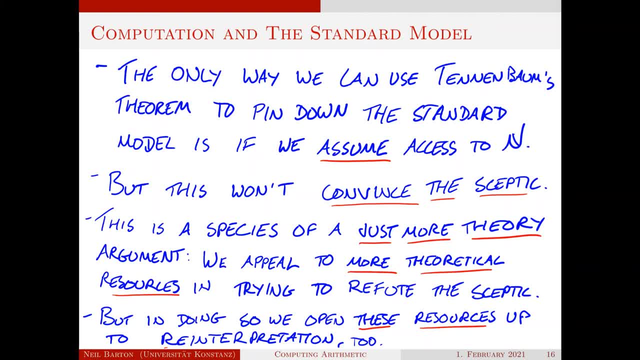 argument. in trying to respond to a skeptic, you better be sure that that more theory you appeal to isn't something that the skeptic can reinterpret. It has to be somehow weaker in flavor than the resources you are trying to appeal to, And I'm not aware of any context in which this kind of argument has really been carried. 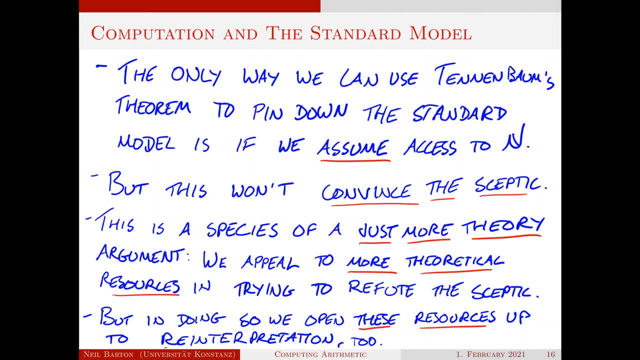 out successfully. In my opinion, in the context of computation, it's pretty clear that this problem of appealing to finiteness is going to be very, very hard to get rid of, if you want to use Tenenbaum's theorem or something similar. 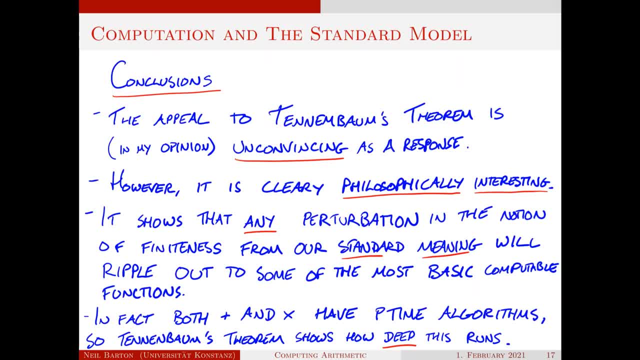 Okay, So Just to sum up and maybe point towards some philosophically interesting ways we might take future study of Tenenbaum's theorem. So I think as a response to the skeptic, Tenenbaum's theorem is unconvincing. This is not my point. as I mentioned, this has been pointed out variously in the literature. 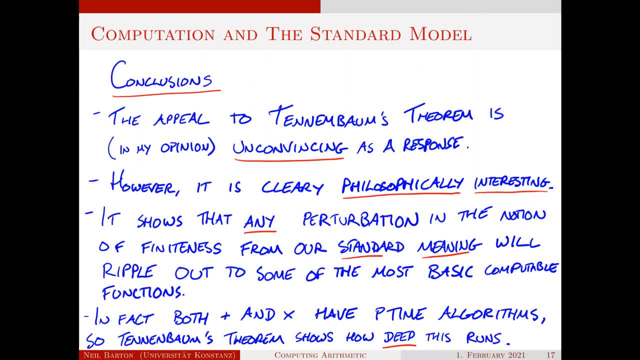 However, I do think Tenenbaum's theorem is really quite philosophically interesting. So, aside from skeptical words, let's assume that we do have a decent access to the natural numbers. I think that's very plausible, And what it shows is that any perturbation in the notion of finiteness from our standard 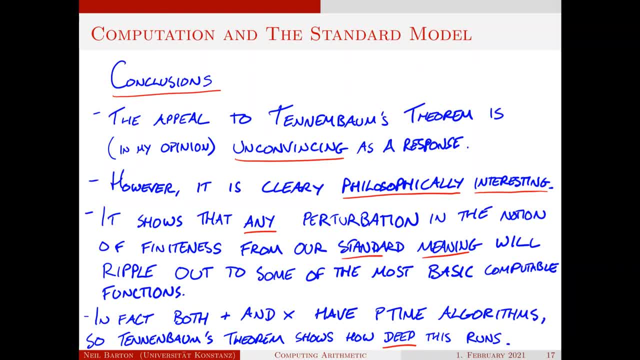 meaning. so any move to some sort of non-standard model is going to ripple out into the really most basic computable functions. So there's no, there's no kind of what it shows you. there's no kind of standard model in which non-standard model which you can move to, in which nonetheless, basic operations like multiplication, 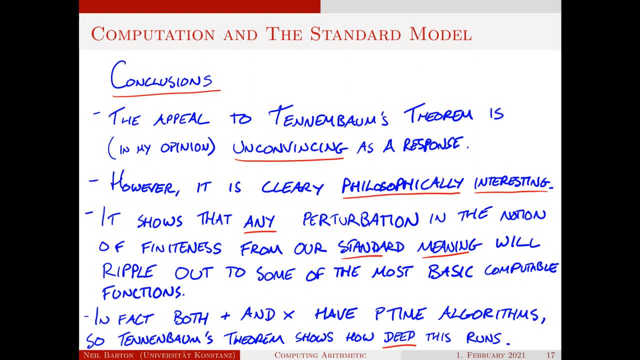 and times remain recursive. Any non-standardness is going to infect even the very most basic arithmetical operations And I think this feeds back- and this has been pointed out by Walter Dean- into considerations about feasibility, for instance. So both plus and times have 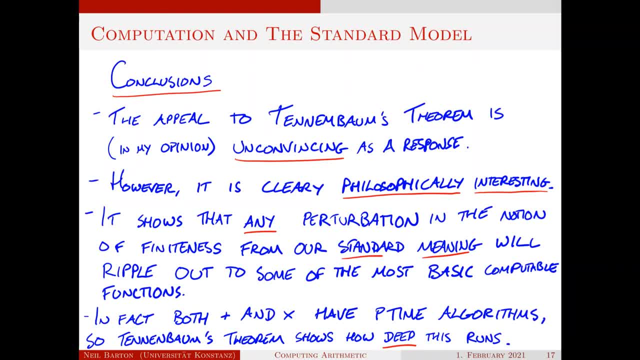 very feasible algorithms. They're both in p-time, In fact, you can do them a bit faster. So what Tenenbaum's theorem is going to tell you is that these very easily computable functions, highly feasibly computable functions, if you move to a non-standard.